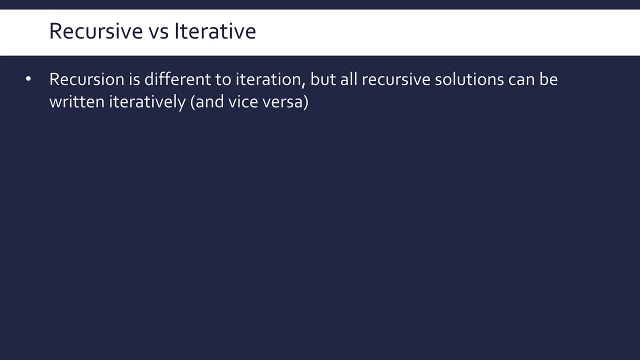 so on the surface they're both very similar, but they are different approaches to solving problems. One thing which is important to know is every recursive solution can be converted to an iterative solution and vice versa, So they're two approaches to solve the same problem. 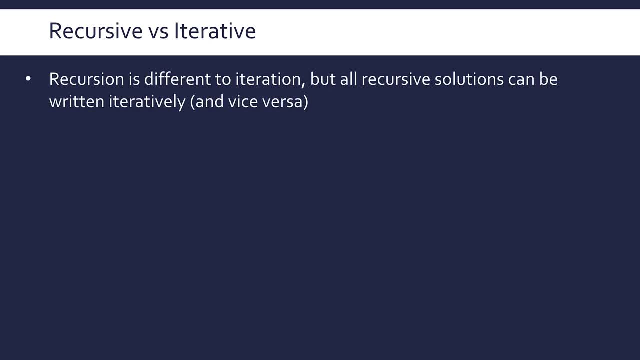 some problems fit really well with recursion, some fit really well with iteration, and so if you try to convert to the other solution, it's going to be different regardless. In these problems we're going to work through the different slights in terms of verbs for this concept, So there's always 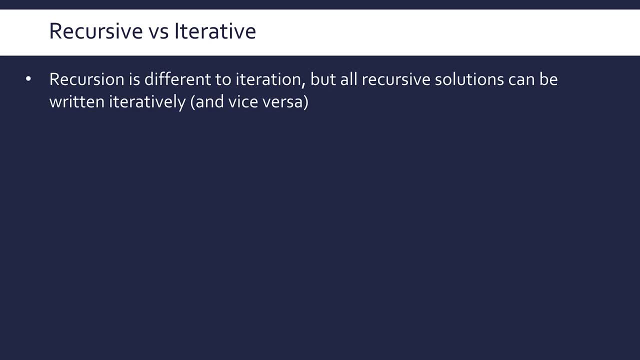 a problem with Trending over tools or so, But for you, i'm assuming, it's mostly a better problem than somehow approach. it might be a bit of a nightmare, but you could in theory. Now just to show you an example which I've used before and is it just a classic in this- which is about factorials: on the left is 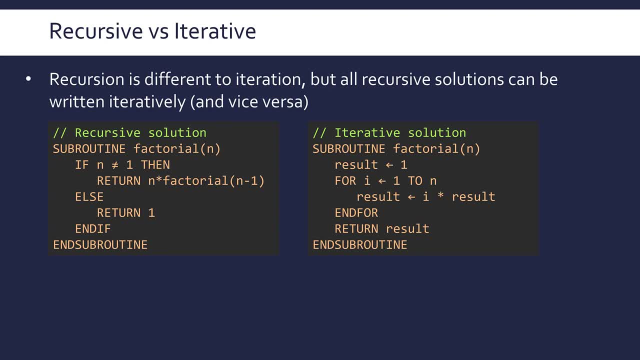 a recursive solution and on the right is an iterative solution. both do the exact same thing. both will give you the factorial of a number, but approach in a different way. so as we, as we run both bits of code, we are going to have repeats. the code is going to repeat, just the order is. 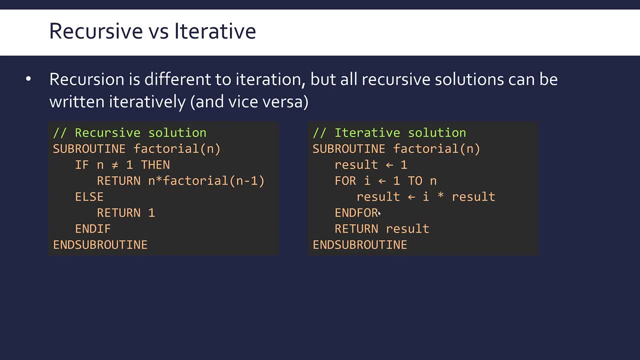 different. the actual repeat in the iterative version is just inside this for loop, whereas the repeat in the recursion is just for the fact we are calling and then returning from different instances of the same subroutine. so it's not quite the same aspect of repetition, although the similarity is that we are repeating the same bits of code multiple times. now both do the same job. 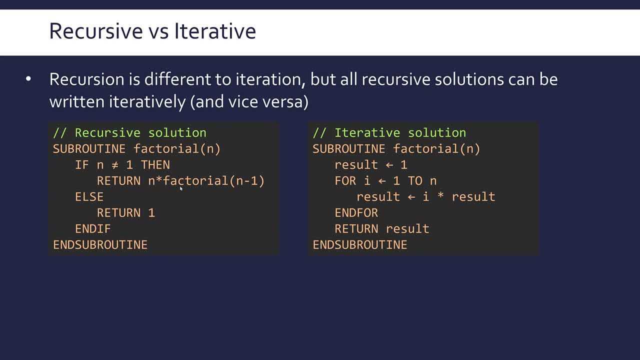 it is down to per personal preference which one you'd want. in this particular case. I personally prefer the recursive solution because in my mind it fits a lot better with the mathematical definition. when you see the maths definition, as I showed in a previous video, you can clearly see how this code. 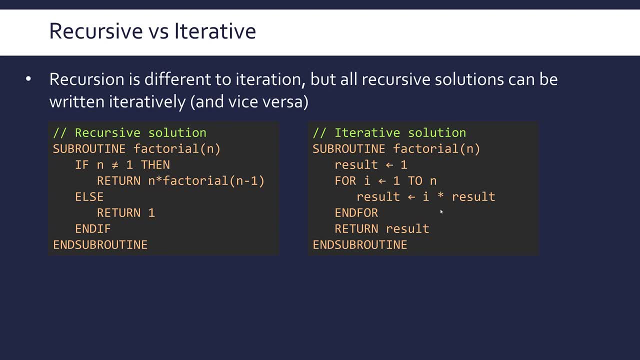 implements those mathematical rules, whereas if you're leaping from the right to a mathematician, they might not fully understand what's going on in this particular bit of code, whereas you'd hope they would at least get the sense of what you're doing on the left-hand side. but ultimately the difference is very. 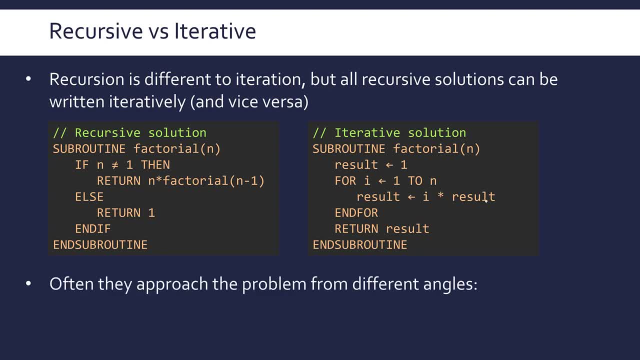 approaching the problem from different angles. a lot of the time- not always, but a lot of the time- iterative solutions will start small and build their way up. so you'll start at the kind of smallest area of your problem and just work your way up until you have your solution. 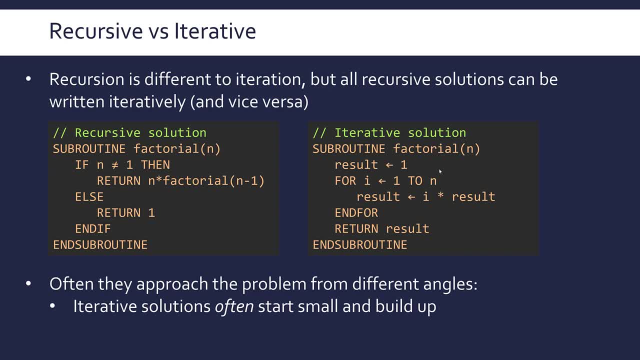 so really a bottom-up approach with factorials. my code here starts with i bing one, and before the increments it gets bigger and bigger until we reach n, and we're just going to. we're just multiplying this kind of cumulative product as we go. I could have done it the other. 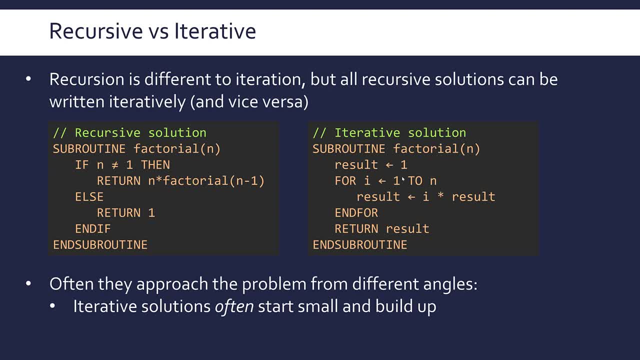 way around, but it tends to work better with iteration if you start small, Whereas recursion, I've found, tends to work better if you start big and then use your general cases to break it down into smaller and smaller problems. So the way the coder on F did work is well. we pass in our 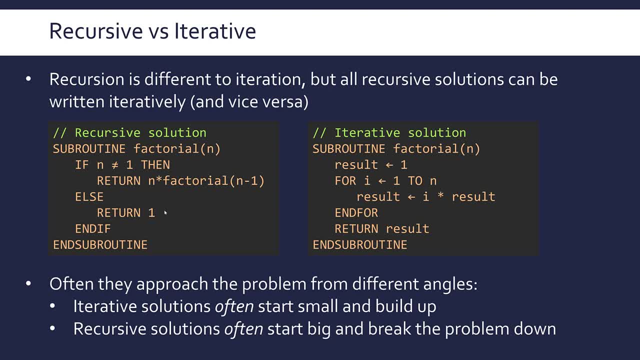 argument for factorial and instead of the solution kind of working its way up towards it, it's going to start calling itself with smaller versions of n, and that constantly calls itself and calls itself and calls itself, with smaller and smaller and smaller versions of n until we reach n is 1. 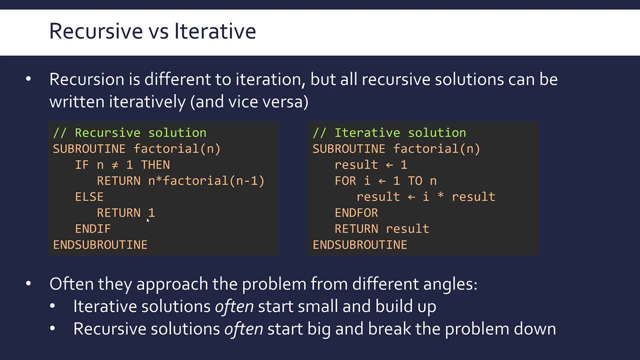 and we reach our base case. So we're starting big and break it down again and again and again until we reach a simple base case or base cases. It works really well for divide and conquer problems, So, for instance, merge sort is a really good example of a usually recursive solution. 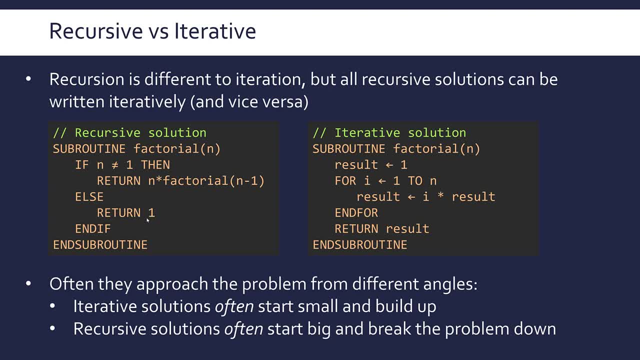 The way merge, sort, works, works on lists is it'll divide the list again and again, and again and again until you've got a list of one item only and then slowly, pair by pair, it's going to sort each pair until the list is rebuilt in a sorted way, And because that's breaking it down going, 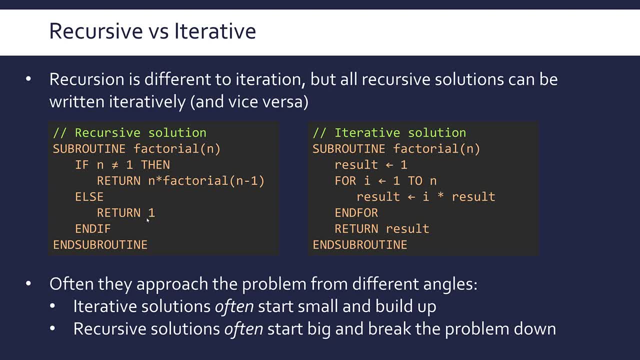 top down. it's a good example of how recursion can fit in really well. If you ever look at an iterative solution for merge sort, which is bottom up, I think it's much more confusing because it kind of goes against the nature of what merge sort. 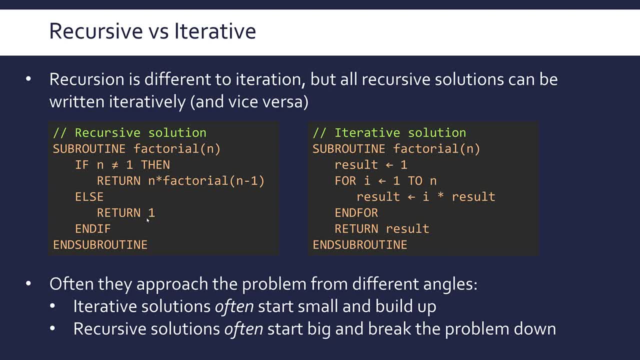 is doing. Merge sort is trying to break down a problem, and so it fits better, in my view, with recursion than iteration, But ultimately both do the same job. it's just what approach you're taking to solve it. So, if I can just do a few more comparison points because I think, just to be as explicit, 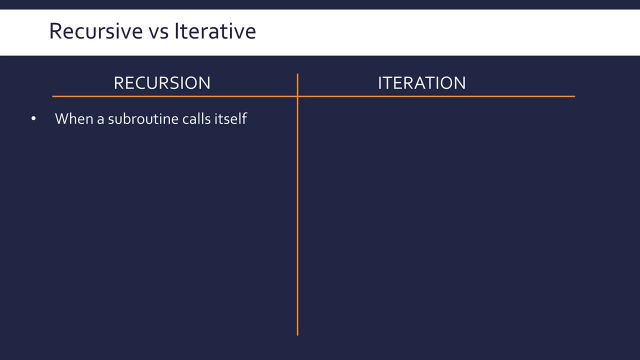 as we can is important. So if you look at code and you want to figure out if it's recursive or iterative, well, if it's recursive, it's when you can see a subroutine, a functional procedural method, Whereas if it's just using for loops while loops repeat until loops do while loops. 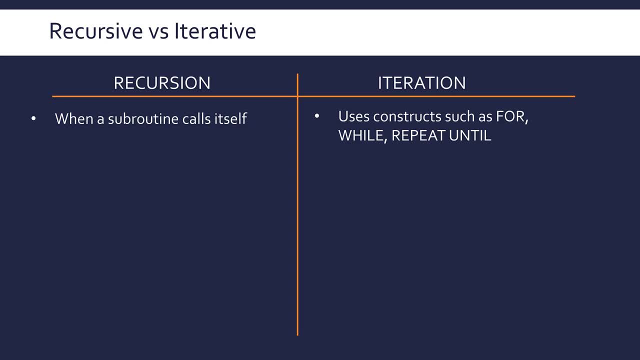 any other version of those. it is using an iterative approach And you might have a combination sometimes, but within a recursive subroutine really it should not have any iteration. Both have problems. of course, Recursive solutions can run infinitely. I've put that in quotes. 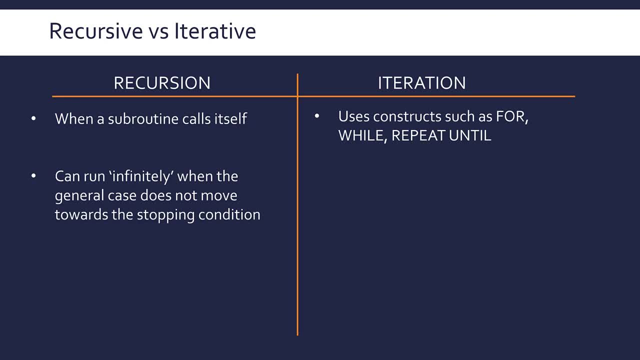 because it's not truly infinite. it's going to crash eventually And it can be this infinite case where you don't actually have a general case which moves you towards the stopping condition. You've got to have a situation where every call of itself moves you closer towards that. 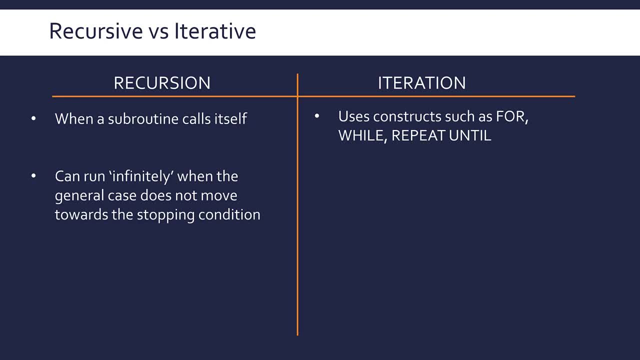 base case which will stop the recursion. So it will be infinite. if you haven't got a well-defined base case, But in reality it's going to crash, it's going to run out of space. you'll have a stack overflow where it just hasn't got memory to deal with all of these pending subroutine. 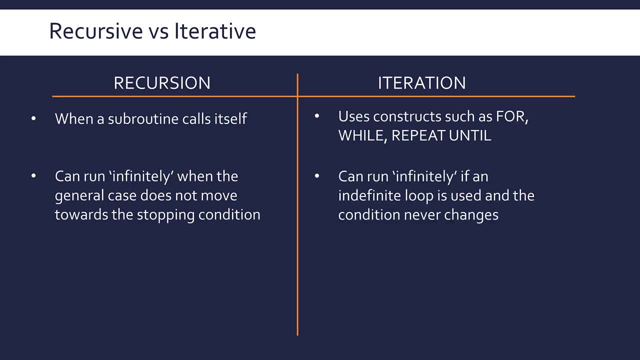 calls And loops. as you will well know, I'm sure, can also be used for recursive subroutines And loops. as you will well know, I'm sure, can also be used for recursive subroutines And loops. as you will well know, I'm sure, can also be used for recursive subroutines. 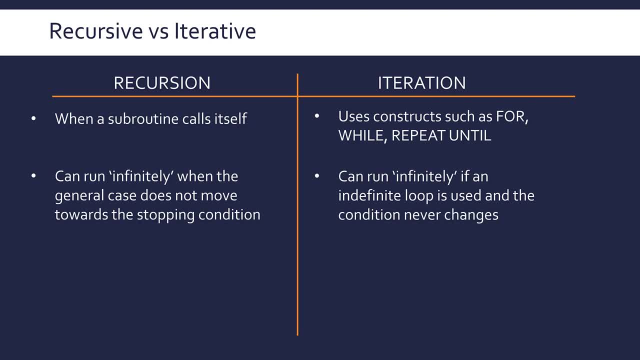 And again, they should all be infinite, not for loops, but while un-repeat, until loops, which are indefinite, could be infinite. Again, I've used that in quotes because it's not truly infinite. of course. it's going to crash eventually or you're going to have to cancel. 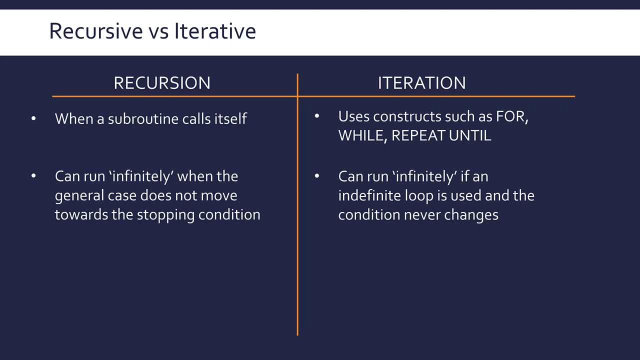 it eventually. It can be infinite if your condition never changes and if you don't use a construct like break which ends it early, The difference being I suppose recursive is a bit more dangerous if it runs infinitely, because it's going to crash And it can be quite a serious. 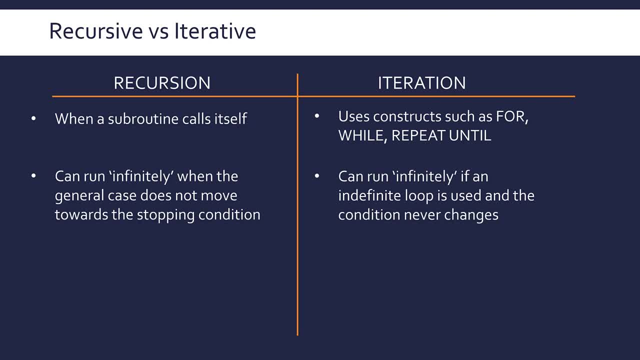 crash in certain cases, cases, whereas iteration it's going to crash eventually, but most of the time it's just wasting your CPU, it's just doing stuff for no good reason. in terms of positives, recursive solutions can and I would say are often more concise and readable than iterative solutions, in particular if the 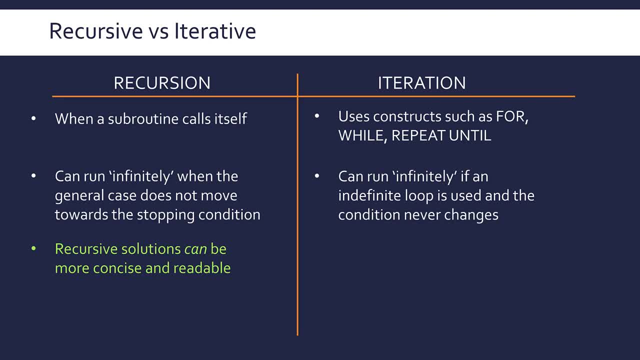 problem lends itself to a divide and conquer approach. something like merge sort fits really well with recursion, and so its solution is more concise than the iterative version. of course you could write some awful code for recursion, but if it's done well, it can be really short and really